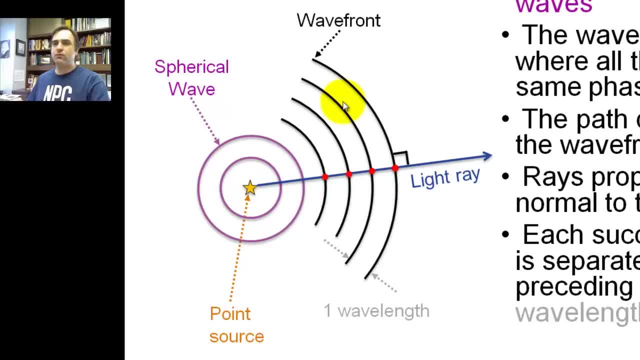 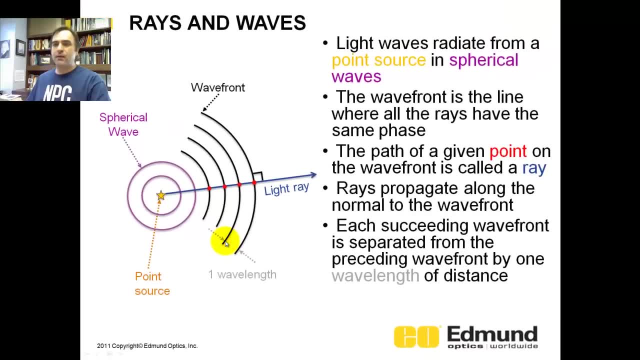 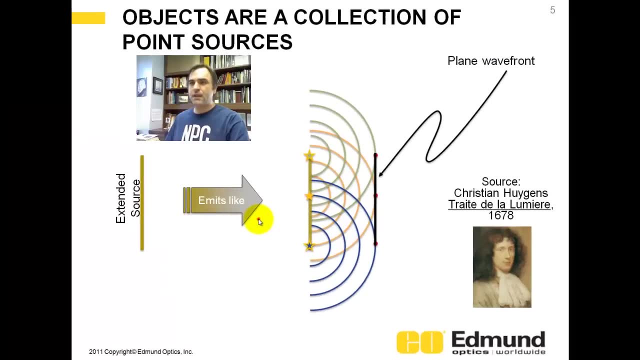 you can represent a point source as a bunch of rays or as a spherical wave front. Now the difference between the peak here and then spatially after some time, t, here that's called a wavelength. So why are point sources important? Here is an extended source, So this is a point. 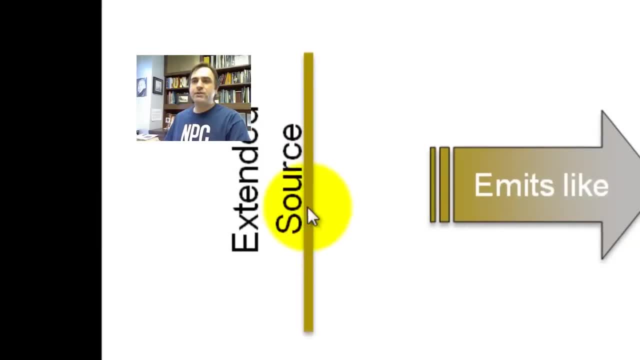 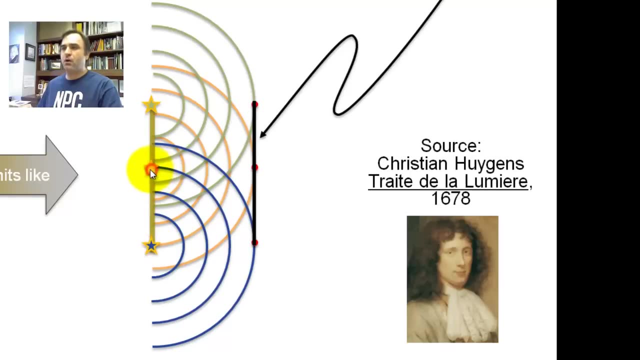 source: a piece of paper, a wall, anything. It's going to emit as if it were a bunch of tiny little point sources here, And what I've done is I've put three small point sources – top, bottom and center. This one in the center is going to emit these golden waves. 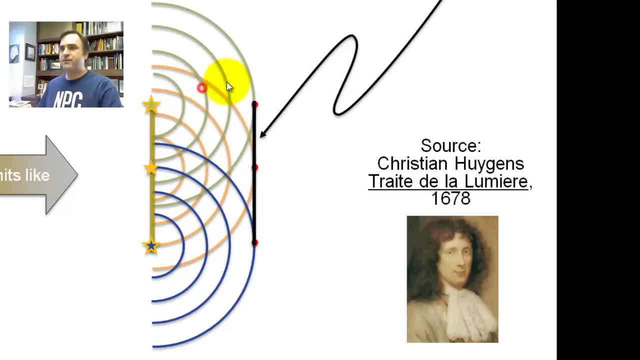 here. This one at the top is going to emit these green waves here And the bottom these blue ones. likewise, If you go out at some time t and you look at the spectrum of light- the same spatial point you know normal to the surface, you're going to see that it. 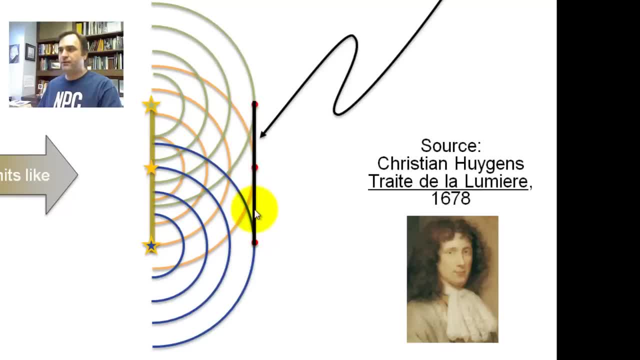 makes a plain wave front. a flat wave front here. This was the fact that an extended source is made up of a bunch of tiny point sources. This was pushed by Huygens back in the 1600s, So this is very powerful. We can model optical systems as a conglomeration of a bunch of 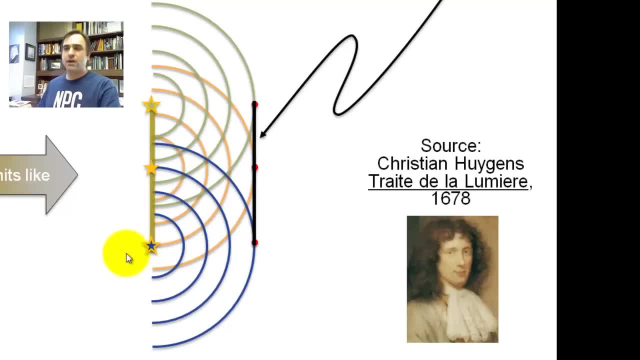 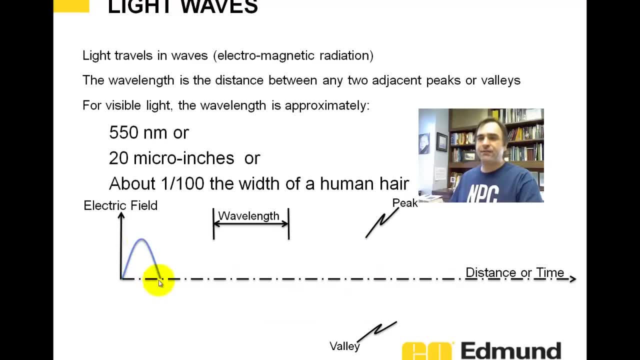 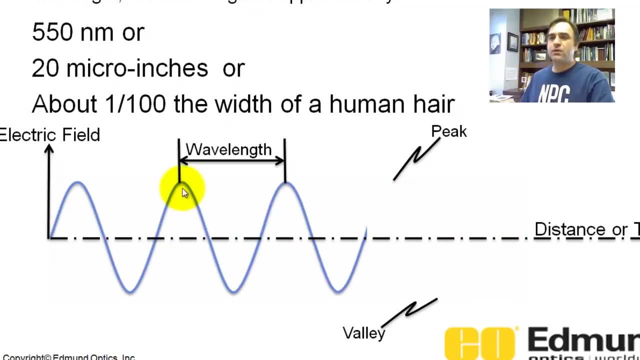 infinitesimally small point sources. So we're going to talk about – a lot about point sources. So what is a light wave? Here is – I'm plotting the electric field as it travels and propagates along a distance or versus time. So you've got peaks, you've 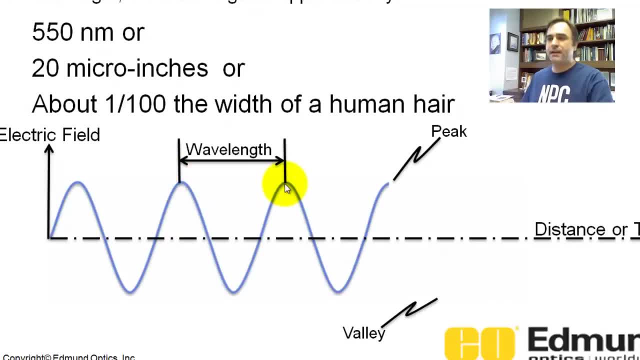 got valleys From one peak to the next peak. that's called the wavelength. Again, from a valley to a valley, that's also the wavelength, Just by way of comparison: visible lights around 500 nanometers or 100 nanometers. 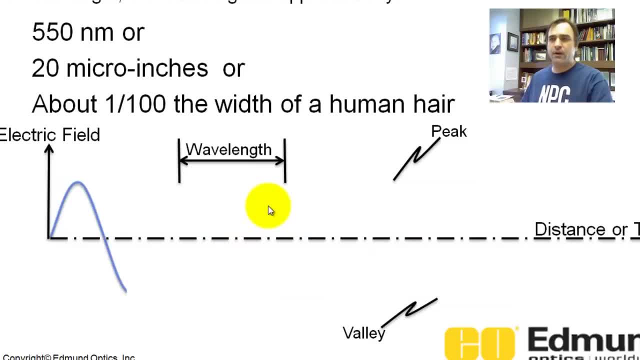 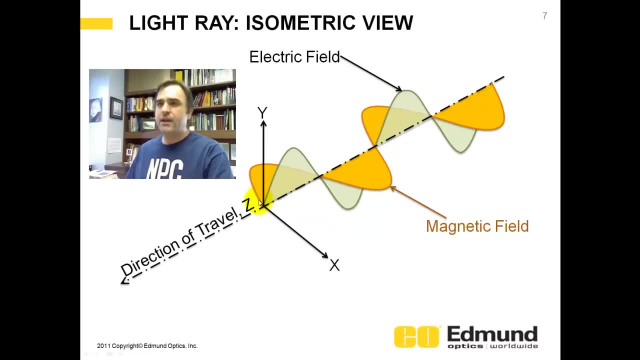 Dad of a light here, A hundredth the width of a human hair. I showed the electric field in the prior chart. This chart I'm showing in three-space. The electric field is here in green and it might be in, say, the Y-plane Perpendicular to it. you're going to have the magnetic field and it's 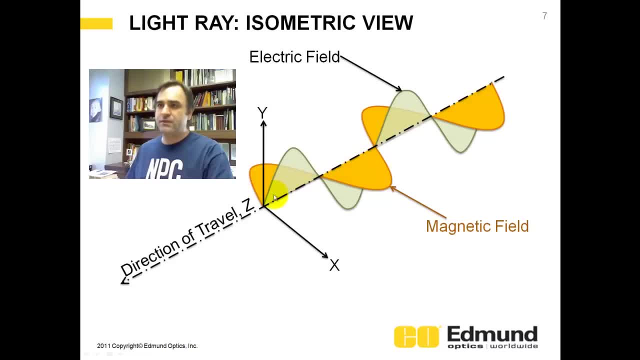 going to be in, say, the X-plane. The direction of travel of this photon is in the Z-plane. Optical engineers like to think of things in terms of the direction of these lines, direction of travel in Z. That's usually the coordinate system that we use. Let's talk. 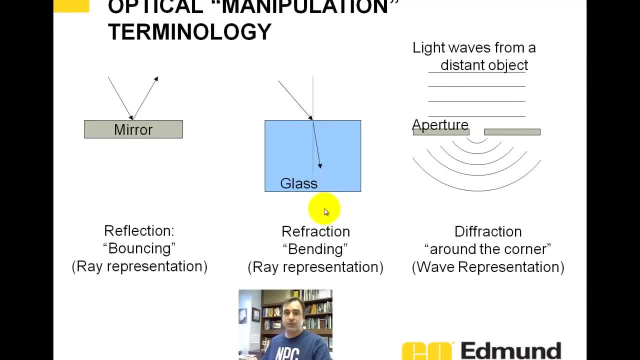 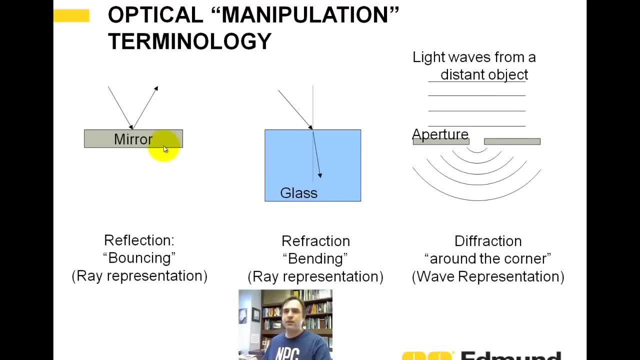 about the different tools we have as an optical engineer to control and manipulate light, And I want to start out with just three right now. First is a mirror and light is going to come in and bounce off of it. This is a ray representation that's called reflection. 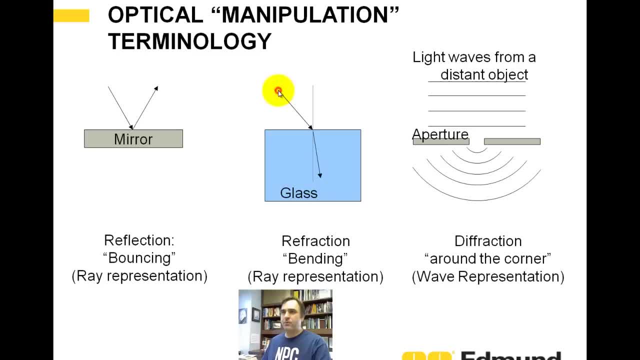 Also we have glass and another ray representation. A light may come in and it's going in the glass and it's going to physically bend the direction of the ray. that's called refraction. We also have how light can bend around a corner, Very similarly like sound waves you can hear. 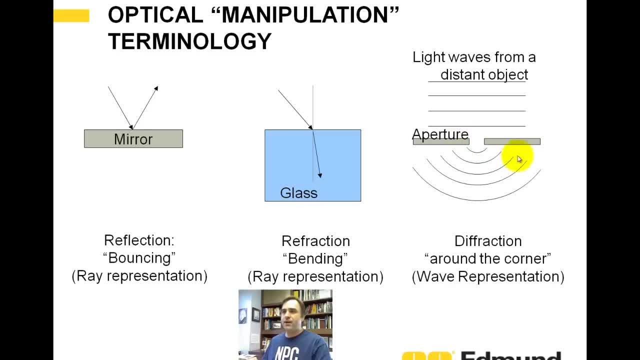 someone from around the corner, Those sound waves. they're traveling around a corner very similar to light. So let's say we have a flat plane here with a hole in it. We've got a plane wave coming in. it's going to hit this hole and then it's going to produce. 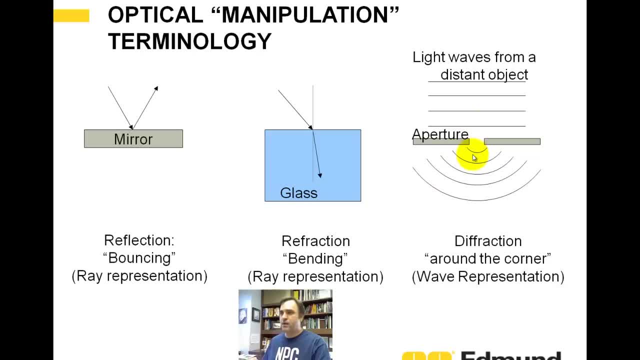 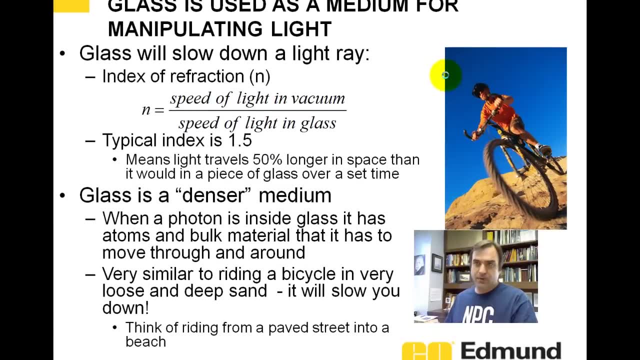 a bunch of spherical waves And that's how light is going to move around the corner. It's going to bend around a corner. This is called refraction. Glass is used as a medium for manipulating light, And glass is going to physically slow down the light. So we characterize. 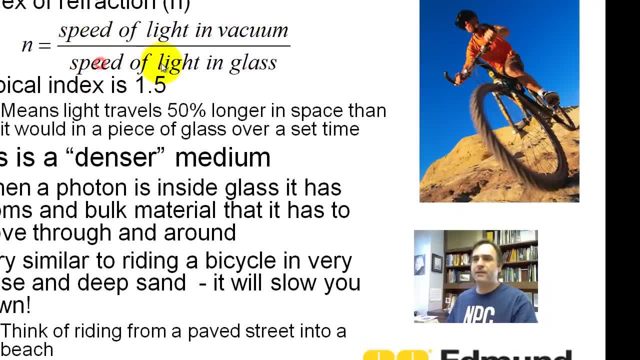 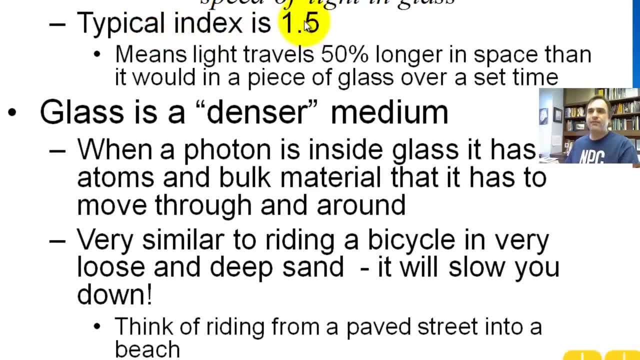 glass by the speed of light in a vacuum divided by the speed of light in glass. For a glass you look out like your window. its index is around one and a half, So that means light is going to travel fifty percent farther in the direction of the light than it is in the 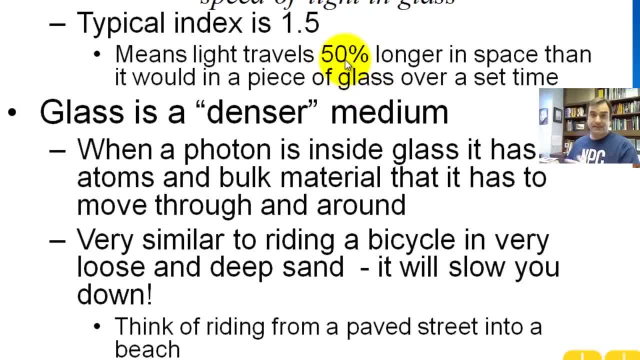 space than it would in a piece of glass for a set amount of time. So glass is a denser medium and I like to think of it as a photon is going into this medium and it's a bulk material. it's got to move through and around atoms. This is very similar to riding a bicycle. 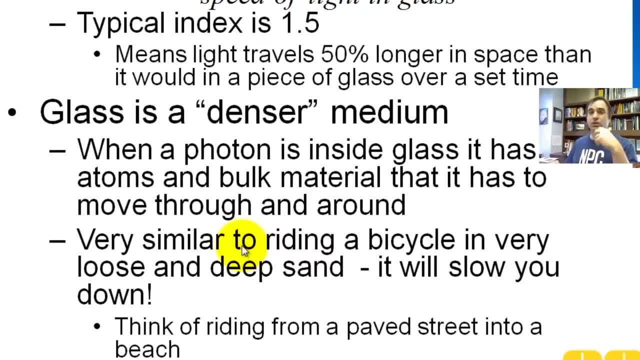 I like this analogy because it's going to give you a good intuitive understanding. Let us suppose you're on a bike and you're riding on a freshly paved road that's very nice and smooth. that's like air. You're going to go into deep sand and that's going to slow you down. That's like glass. 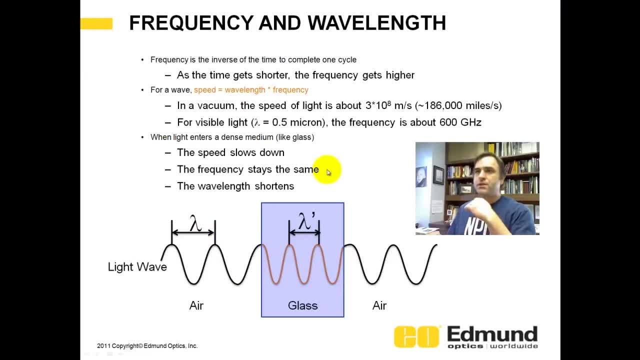 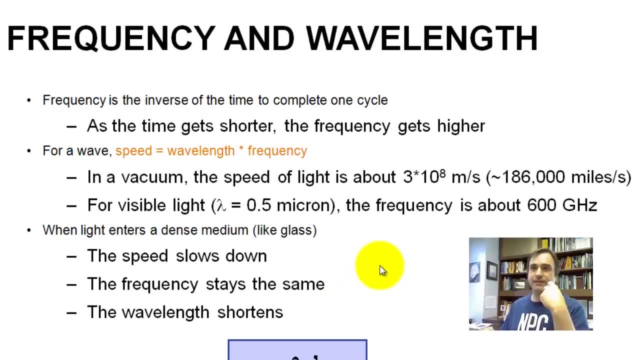 deep sand, like at a beach. So frequency is the inverse of the time to complete one cycle. So as time gets shorter, the frequency gets higher. For a wave, for a photon, the speed is proportional to the wavelength times the frequency. So in a vacuum a photon is going. 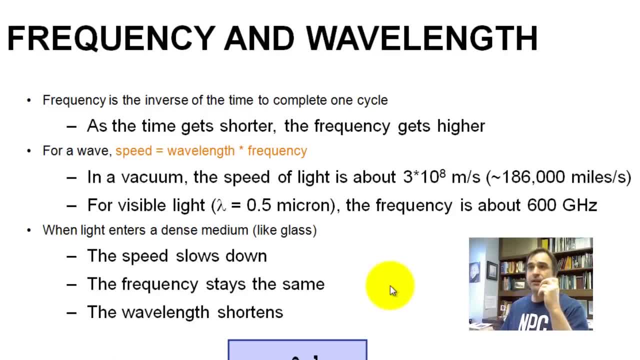 to travel at about three times the speed of a wave length. So the speed is proportional to three times 10, to the 8 meters per second For visible light, then its frequency is 600 gigahertz. When light enters glass, the speed is going to slow down The frequency. 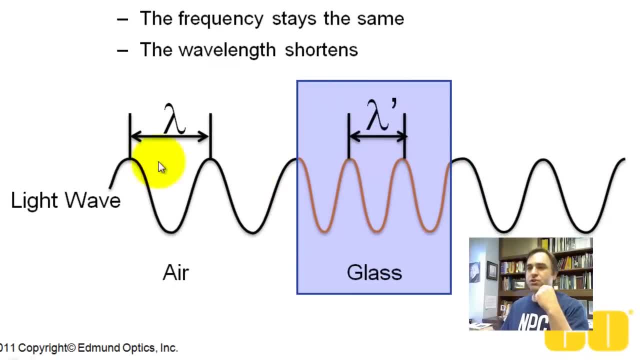 stays the same. so the wavelength has to shorten And that's shown here. You have a wave, you know a light beam coming in with a certain wavelength. It's going to hit the glass here and you can see the wavelength is going to actually get shorter and then continue the 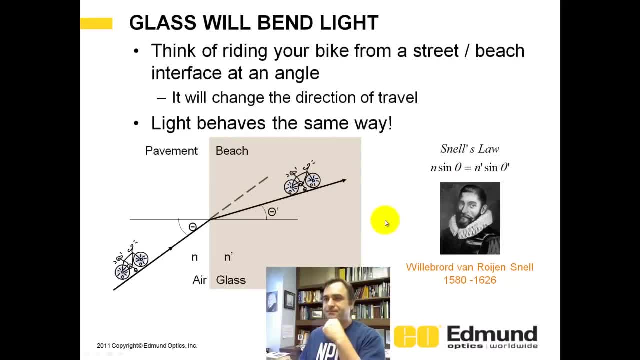 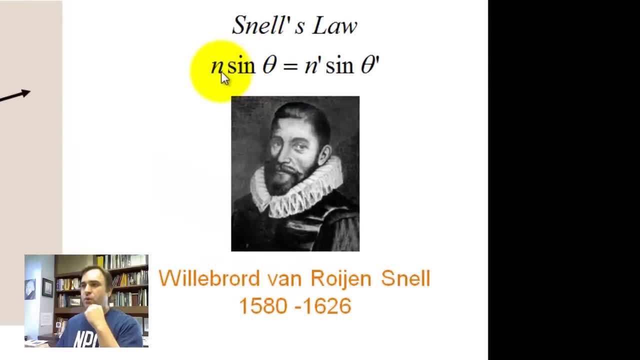 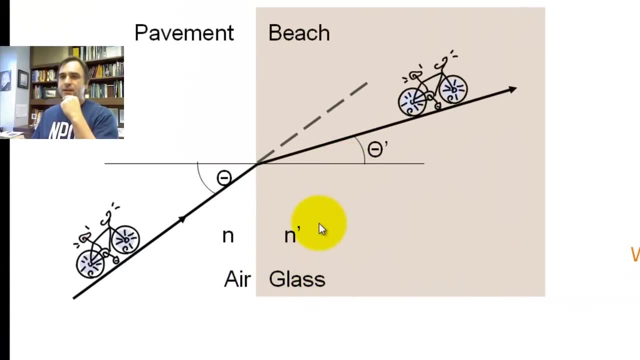 same original wavelength when it comes out into air again. So how is light bent? It's characterized by Snell's Law. It's this equation: N sine theta equals N prime sine theta. prime: Unprimed is in air, Primed is in glass. So the analogy: 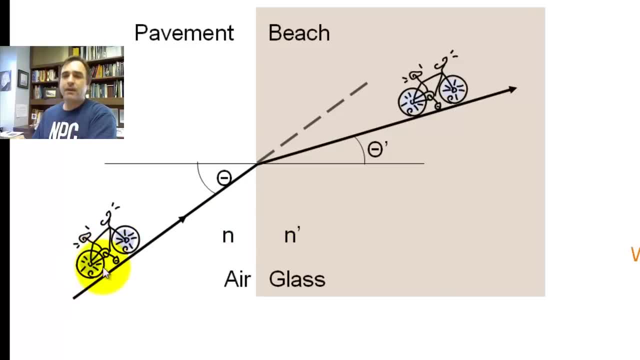 back to the analogy of riding your bike. you're riding your bike on pavement. Now and note: if you ride your bike perpendicular to the pavement beach interface, you're not going to change any direction. If you ride your bike at an angle, your right side of your 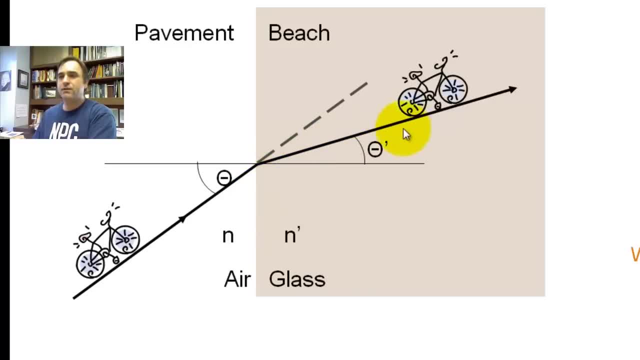 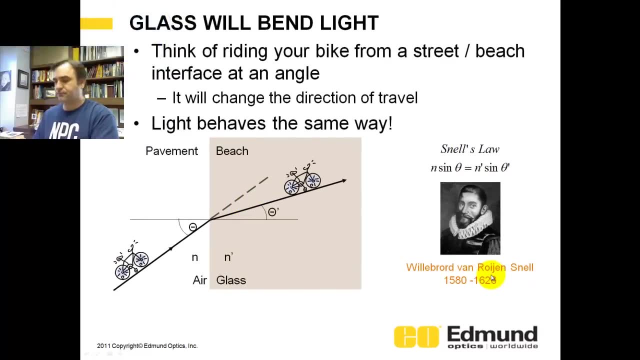 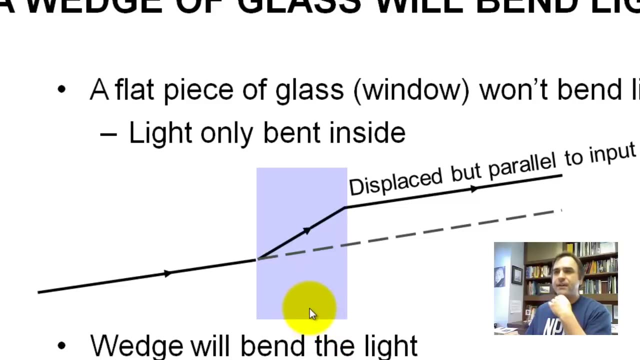 of the bike is going to enter first and it's going to pull the bike to the right, And that's what is happening with a photon. That is why light is slowed down. So that's in a medium. Glass doesn't extend for infinity. You've got windows, or, as we like to get fancy. 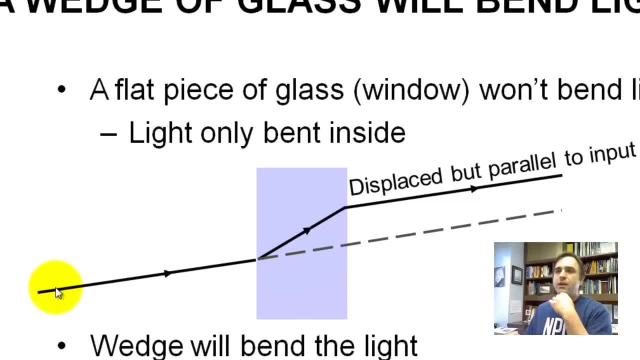 a plane parallel plate like here, You have a ray that comes in When it leaves this window it's not going to bend at all. It's going to be displaced because there's bending going on within the glass and this displacement is proportional to index and thickness. On the other hand, 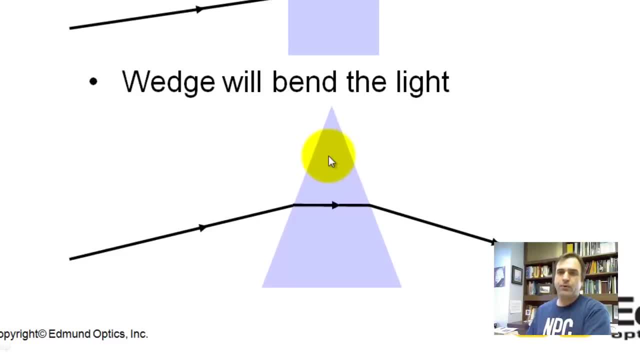 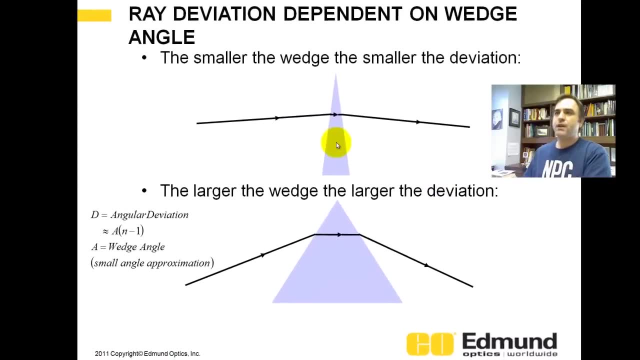 if we put a wedge in the window or a prism, you're going to deviate this beam. here You can see it's physically bent. So this apex angle up here we call it A. That's this A right here The larger.